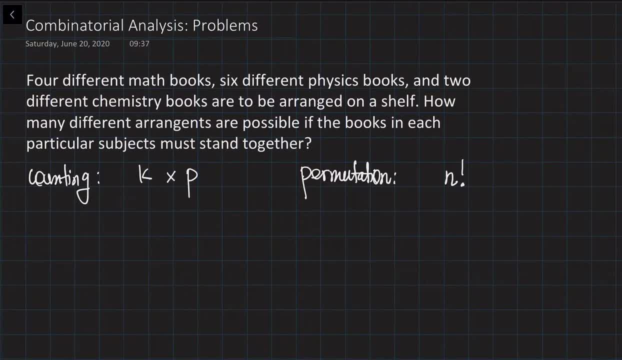 should stand together. So we are going to split this problem into the two different levels, into the levels of the books, rearrangements of the books and also rearrangements of the blocks. So let us create the three blocks. So we are going to have one block. 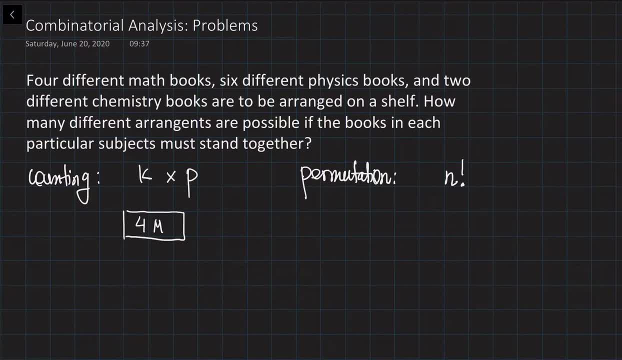 with the four math books. So we are going to have another block with the six different physics books And we are going to have the third block with the two different chemistry books. two different chemistry books. So the number of the rearrangements of these four math books, different math books, is. 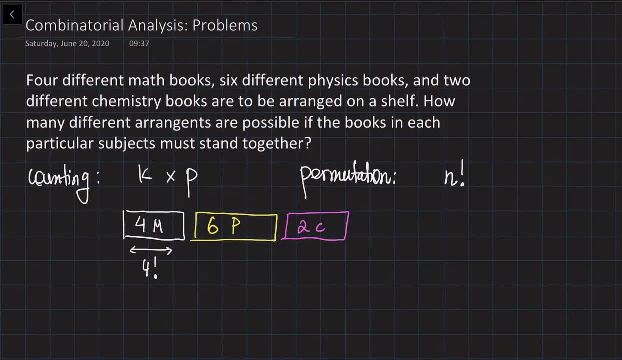 going to be equal to the four factorials according to the permutation rule, And the number of the rearrangements of these two chemistry books is going to be equal to the two factorials. So let me explain to you. what does it mean, this t factorial? 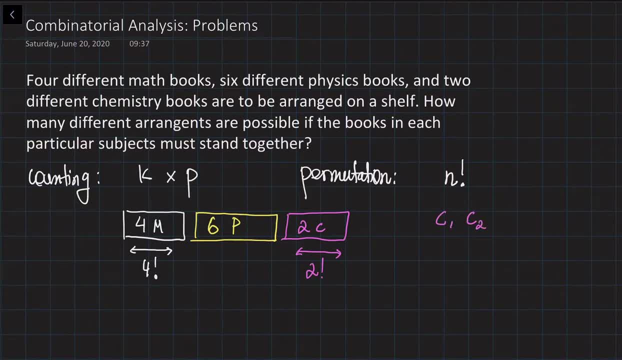 So you have two books of chemistry 1 and chemistry 2, right, And you can arrange them like this, or you can put them as a chemistry 2 and chemistry 1.. So that is why you have like two factorial cases of the rearrangements, or simply two rearrangements. 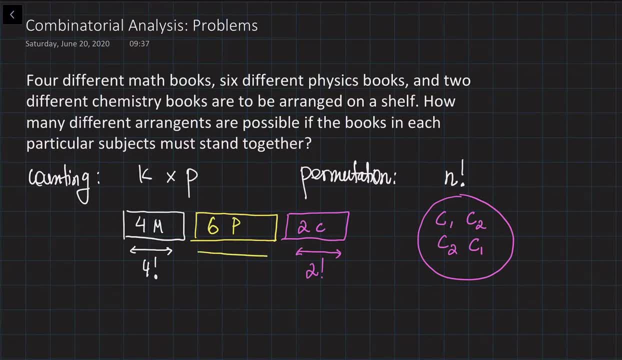 And if you have six physics books, the number of the rearrangements of the six books is equal to the six factorials. So then the number of the rearrangements, in this order in one row, is going to be the multiplication of the four factorials to the six factorials to the two factorials. 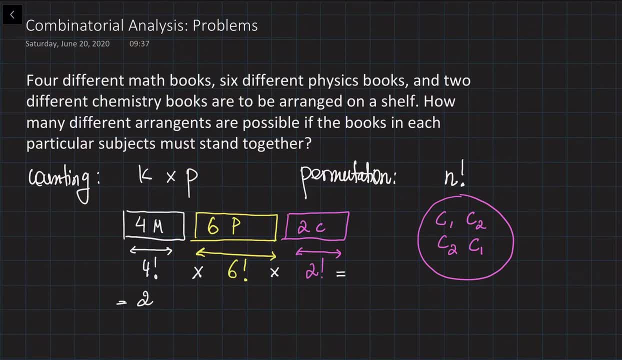 So let's do the calculations here. It's: four factorials is equal to the 24 times six factorials is equal to the 720, and the two factorials is equal to the 2.. So if we calculate this, it's going to be equal to 34,520. 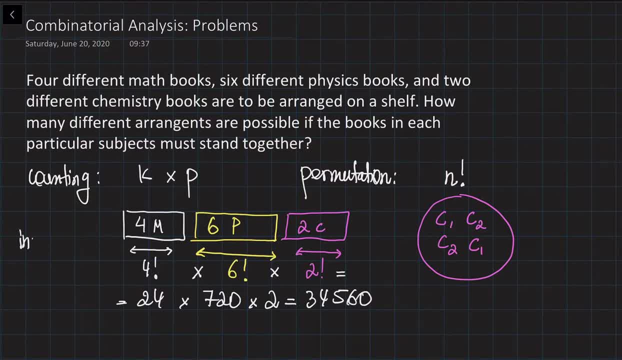 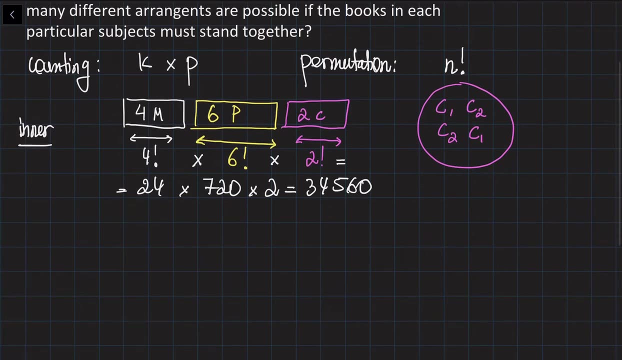 So this is kind of the inner level. If in your bookshelf the math books coming first, then the physics books are coming, then the chemistry books are always coming, then you're going to have 34,560 different rearrangements of this book. 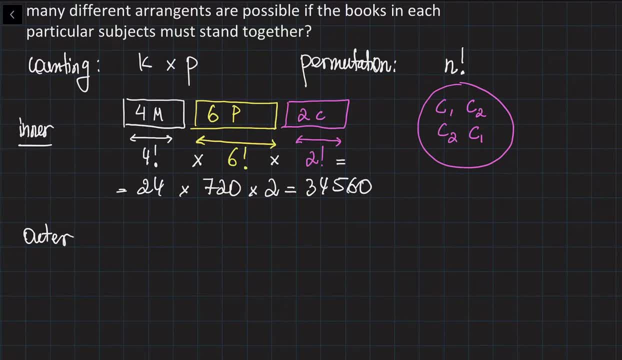 Now we need to look to this from the outer perspective. Basically, I would like to just move the block. So, for example, I would like to put the math books just after the physics, Or the physics books just after the chemistry books. 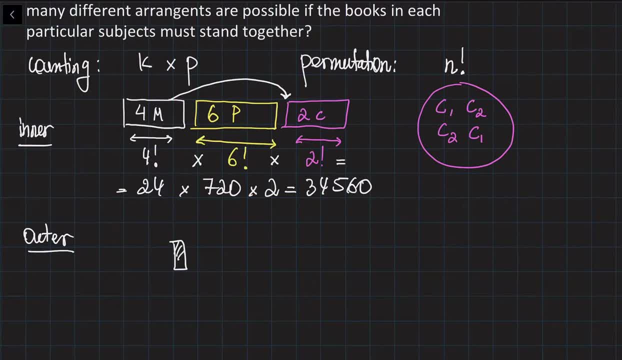 So now we need to look to this from the perspective of the blocks. So you have the white blocks of the math books, You have the yellow block of the physics books And you have the pink block with the chemistry books. right, 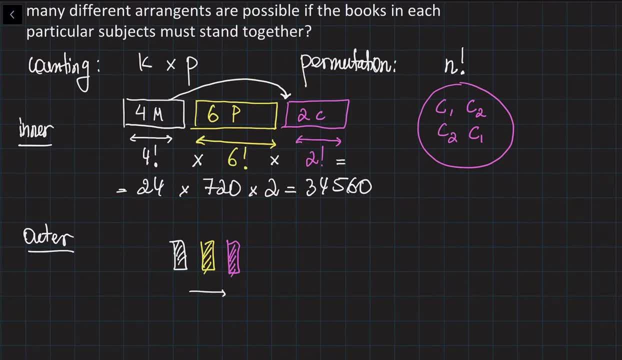 So you basically have three blocks. How many rearrangements are possible? So again, we need to use the permutation rule. If you have three different items, the number of the rearrangements of the three different items is going to be equal to the three factorials. 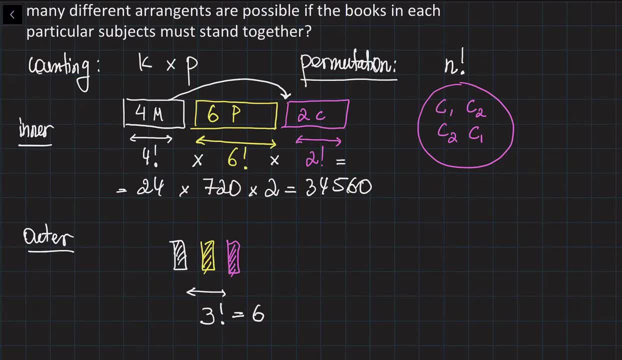 So there are six different rearrangements. So I would like to give you a couple of rearrangements. For example, you can put white yellow, pink, Or you can also put the white pink yellow. You can put the pink white yellow or pink yellow- white. 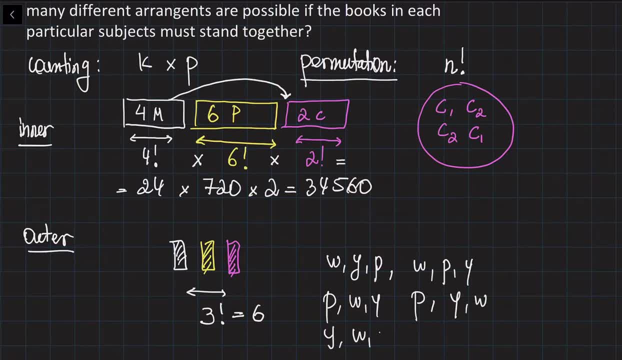 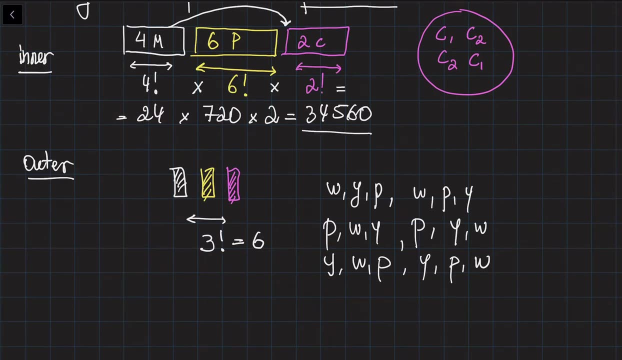 You can put the yellow- white- pink or yellow pink- white. So there are six different rearrangements. There are three different rearrangements of the three blocks. So for every rearrangement of the blocks you have 34,560 cases of the rearrangements of the books. 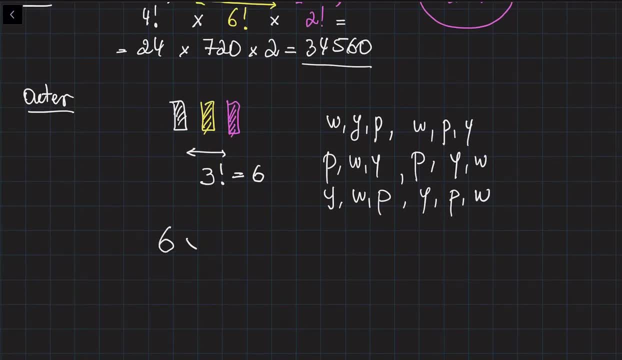 So that is why the number of the rearrangements in total is going to be six times 34,560.. So let me multiply this, It's going to be equal to the 270,360 rearrangements. So this is the solution for this problem. 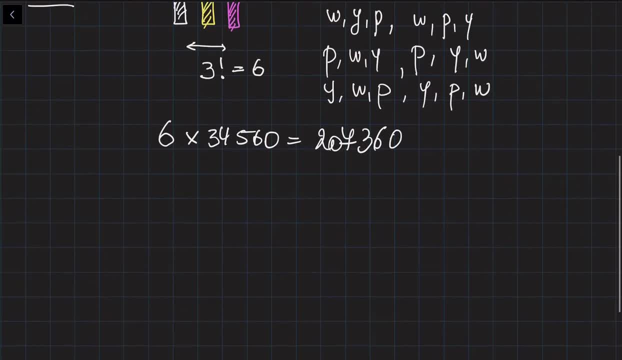 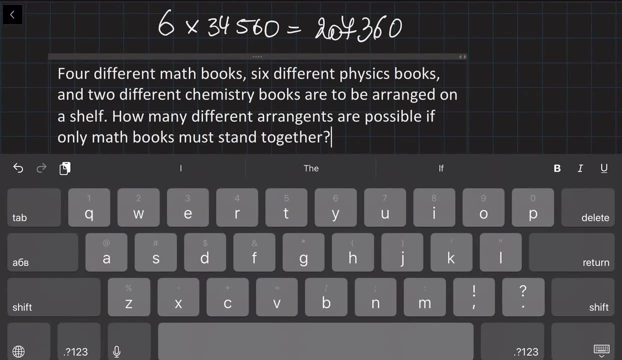 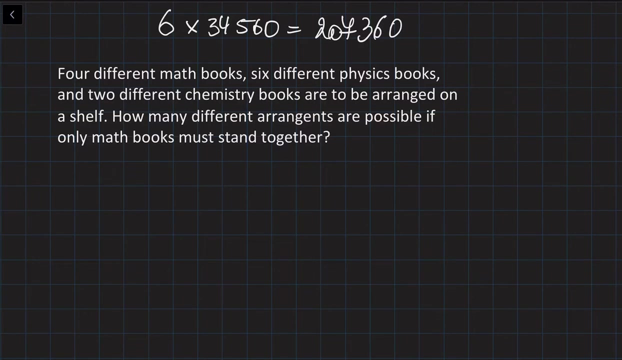 We are going to solve another problem which is going to be very much similar to this one. So again, four different math books, six different physics books and two different chemistry books. We need to find the number of the rearrangements where the math books must stand together only. 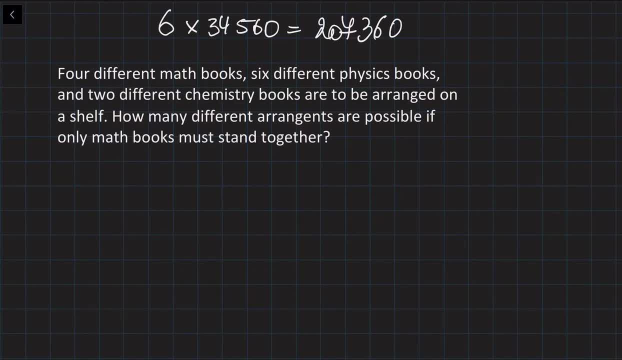 So it is not necessary to make a block. We don't need blocks for the chemistry books or to the physics books. Only we need to have the block for the math books. So in this case I would make the two blocks. 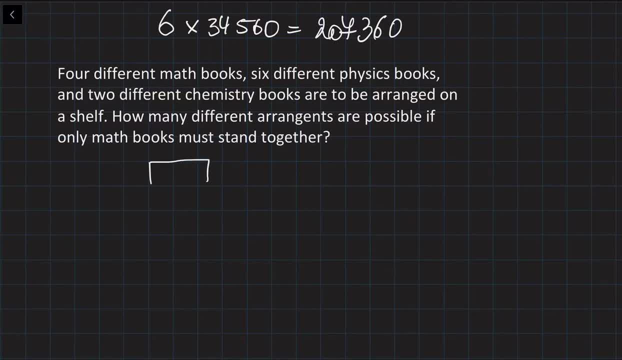 Basically one block with only four math books and another block with all the other books. So how many all the other books we have? We have six physics books and two chemistry books. Basically eight others, right, So eight other books. 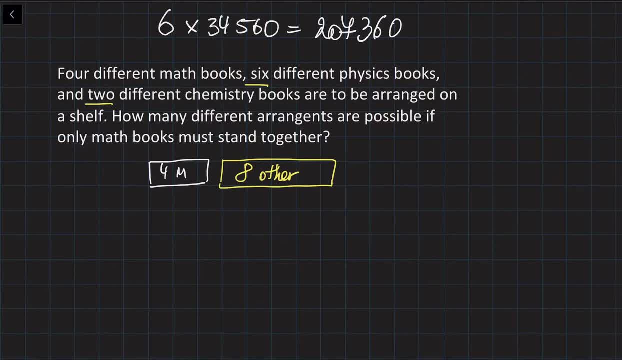 So now what we need to do is, if we put all ways, the math books first, then all the other books, how many rearrangements we have? So basically, in this case like inner arrangements, right, Inner arrangements. 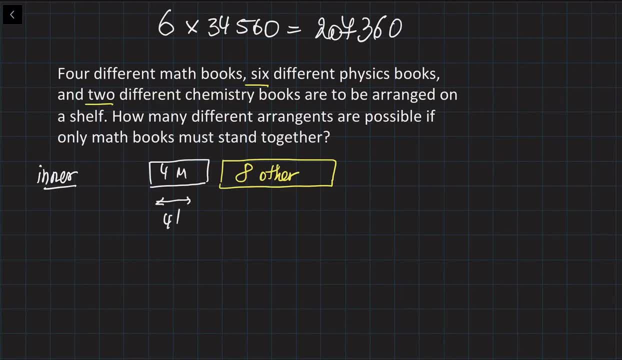 So the four math books are going to be arranged in four factorial different ways And the eight other books are going to be arranged in the eight factorial cases. So the number of the rearrangements of all the books in this one row, where always the block of the math books are coming first. 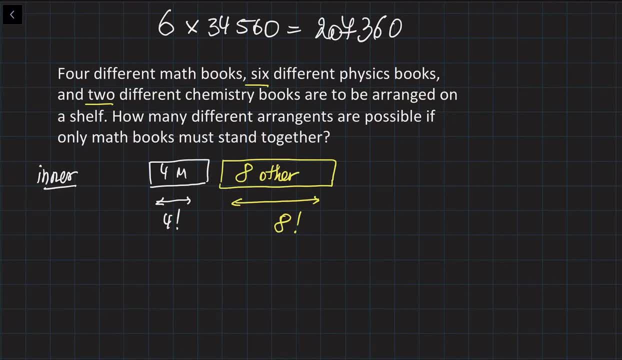 and all the others are coming to. the next is going to be the multiplication of the eight factorials to the four factorials. So let me write this down: So 24 times the eight factorials is going to be 40,320.. 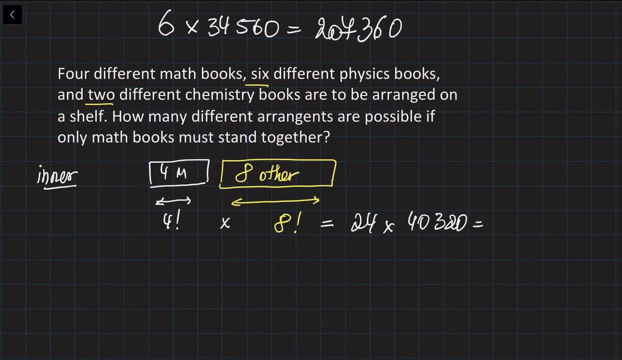 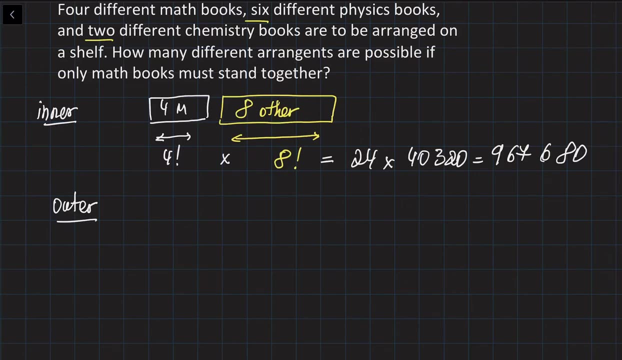 If you multiply this to the 24, it's going to be 967,680.. So now we need to look to this from the outer perspective. What does it mean? It means that you have eight books, So one book, second, third and so on. 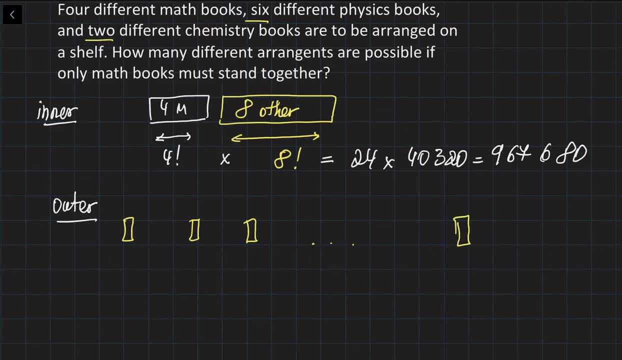 Eight different books. So you can put this block of the math books to the beginning. So one block of the math books to here. But at the same time you can put this block with the math books to here, Or to here after the second book or after the third book. 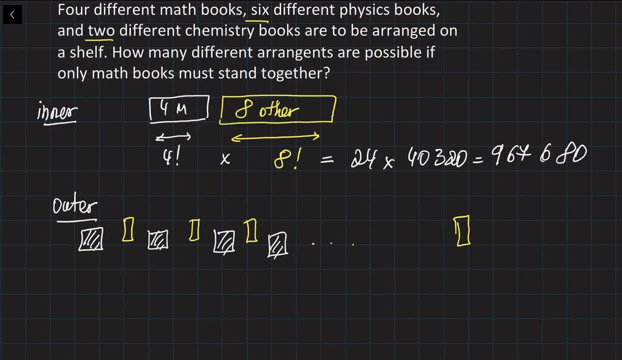 Basically three other books, then the block of the math book and then other five books, Or to here or to here. So since you have, like one, two, three and so on, eight different books, then the number of the positions to put the block of the math books is going to be equal to the nine.